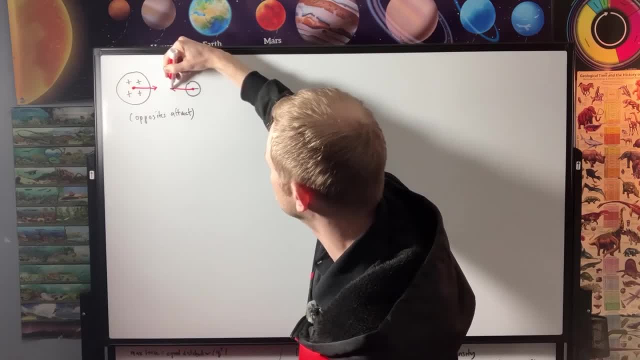 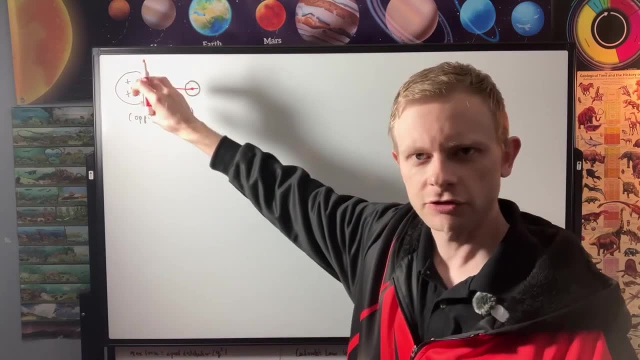 And there's going to be another one over here pulling this direction, coming from that one, And they're going to be equal. Notice that. So just because there's a lot of charge on this one doesn't mean that you know there's any kind of imbalance. 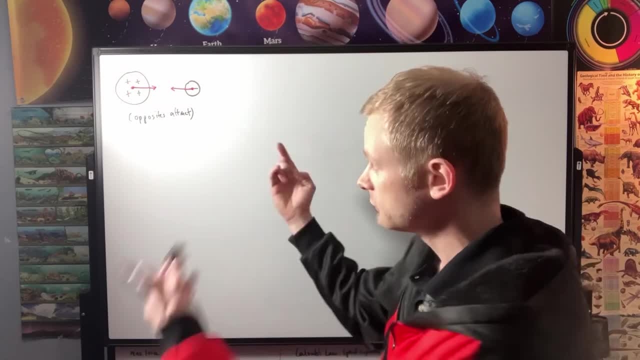 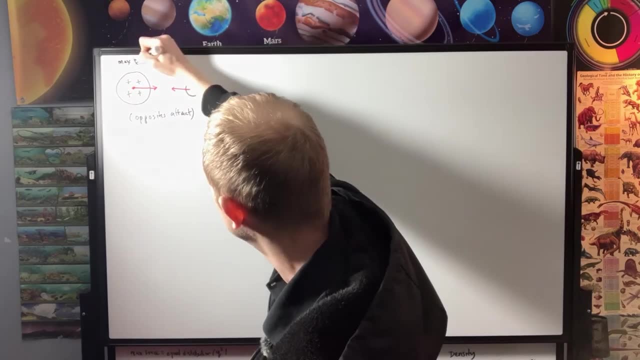 Just like Newton's third law, these two forces are going to be the same, And it turns out that the maximum force that we can possibly get from this right between these two things, the max force, is going to be the equal distribution of charges. 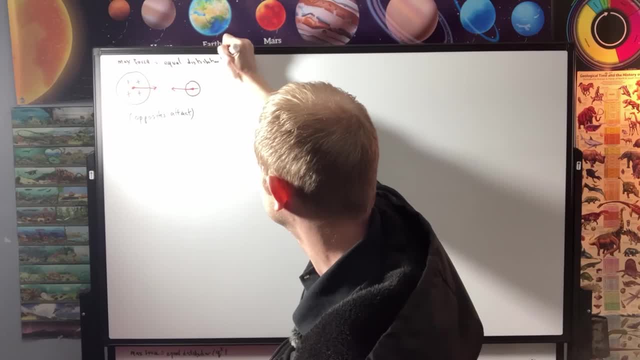 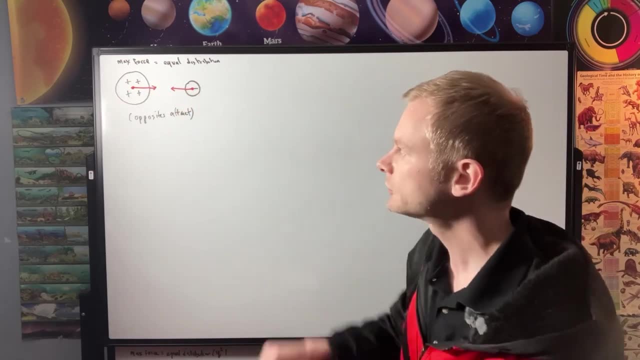 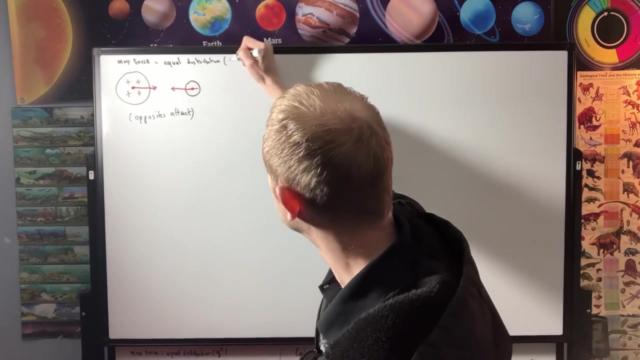 Equal distribution of charges. So notice how these charges are not quite balanced. If we were to give them equal distribution, then they would have the most powerful force between them. That's just what that means, right there. We can represent that as Q squared. once we get into the math. 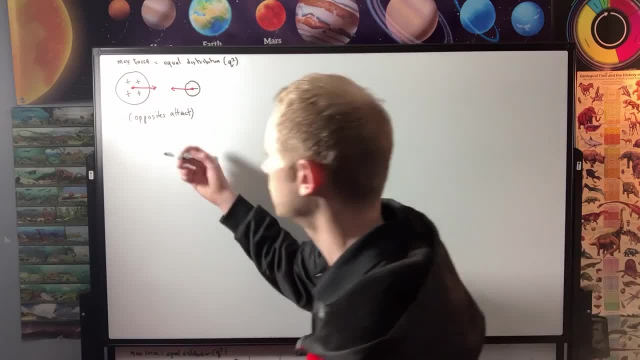 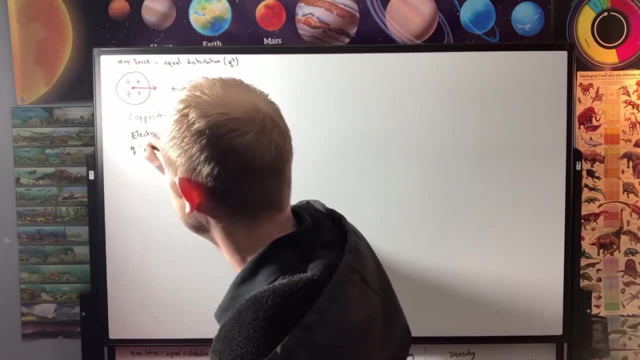 It's going to be equal charges on both sides. Let's figure out what this electric charge is, that we're talking about Electric charge And that's just going to be described by this Q equals, And we're going to have to figure out the difference between the number of protons and electrons in a particle. 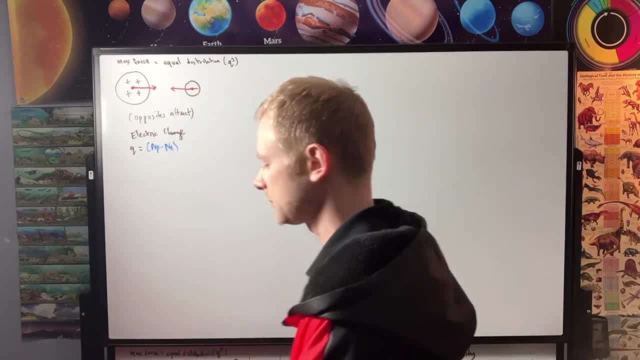 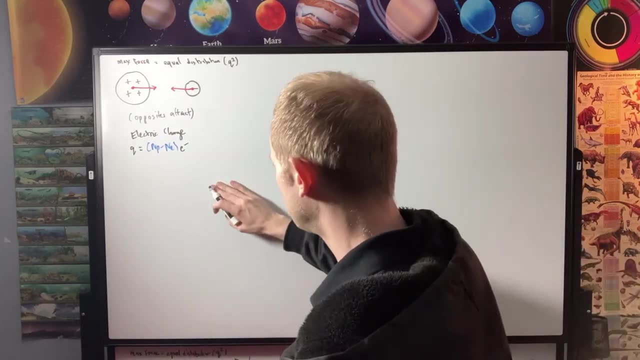 So we've got NP minus NE to represent that, And then we can also multiply that by this E negative, which is going to be the electron charge. That's going to be our little formula, And it turns out that if we have a negative charge, that means we have more electrons. 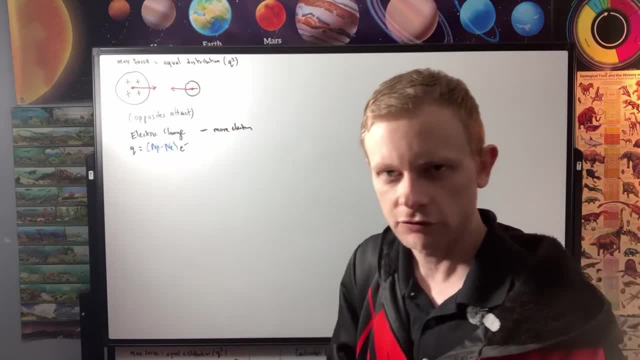 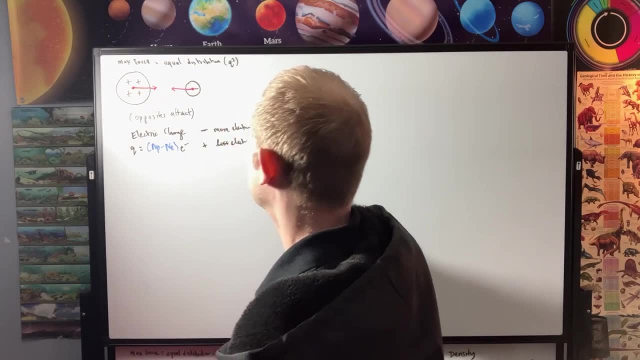 That's because the electrons are negative, And so if you have more electrons you have a negative charge. And so it makes sense that if you take away the electrons, you get less electrons, Then you have a positive charge. You have more protons, you got more positive charge. 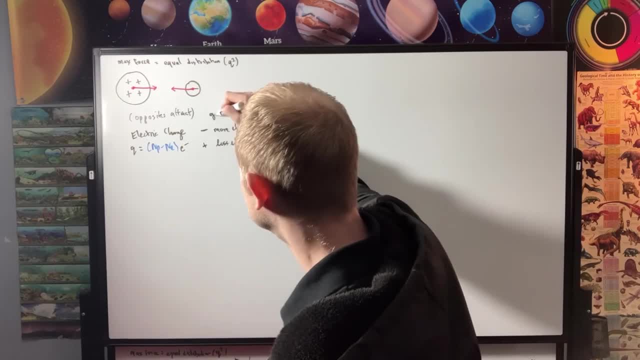 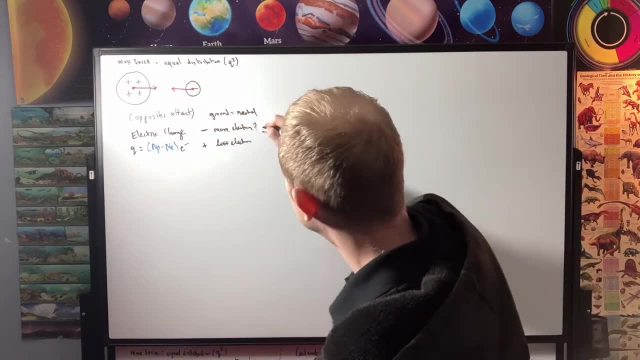 OK, great, Now the ground is neutral, So that's something to keep in mind. Ground is neutral, That's essentially just zero. Now, if you're trying to pull these electrons back and forth from each other to rip them apart, 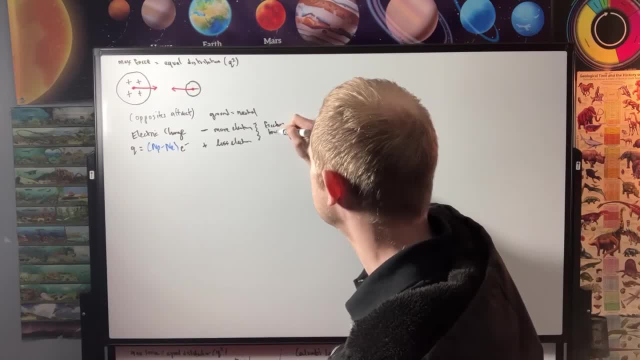 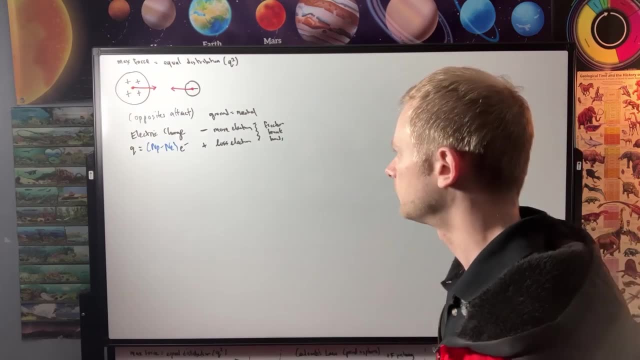 the best way to do that is going to be through friction. These things tend to break bonds, those little chemical bonds, And so then you can rip those electrons apart and kind of transfer them between things. This is just kind of how charges can transfer. 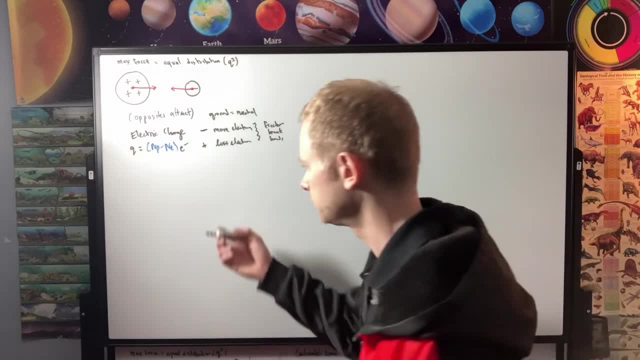 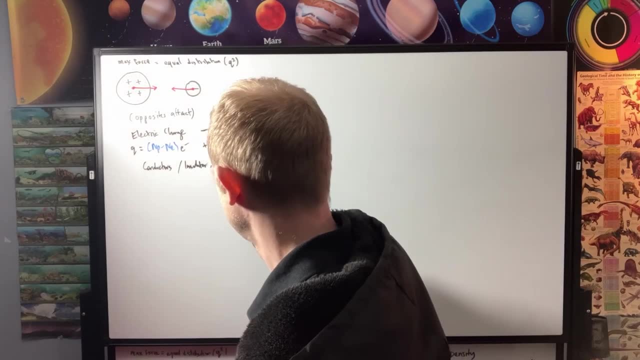 There tends to be two types of compounds in the world. One is going to be the conductors And the other one is going to be the insulators. So conductors are more like metals and stuff. Those things conduct electricity. That means that the charges move. 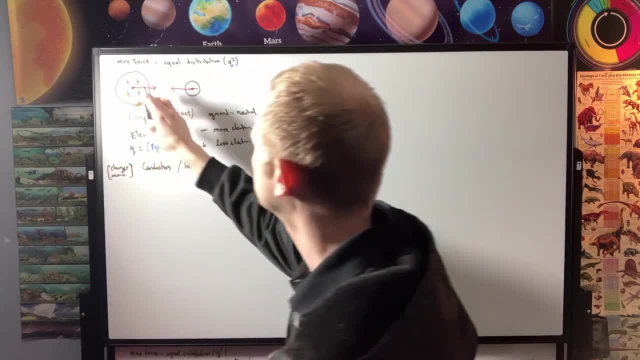 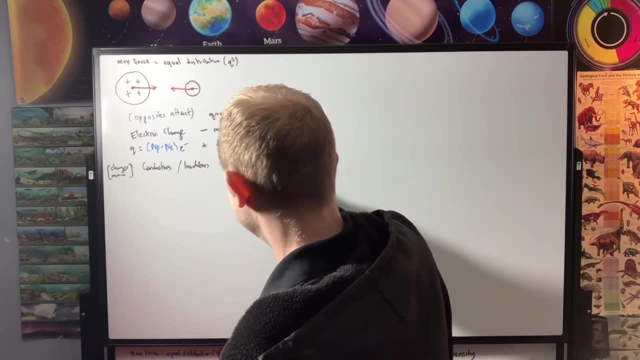 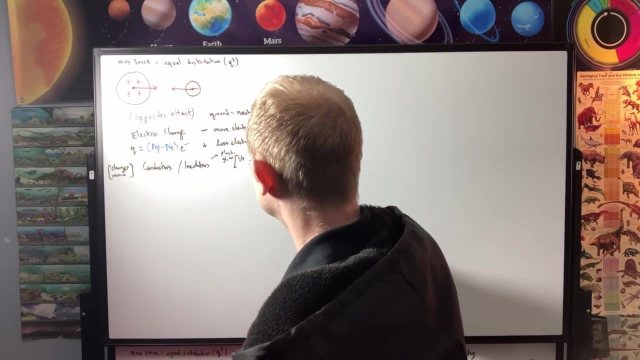 Charges move around, So that means those little pluses and minuses, those things are just going to go, move around and basically just travel. So on the insulator side, though, there's going to be stuff like plastic glass, These things are going to have a static charge. 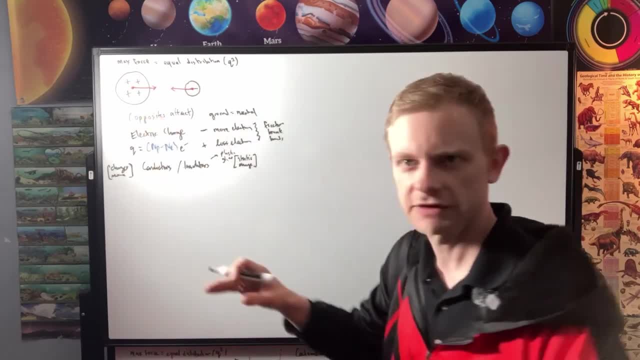 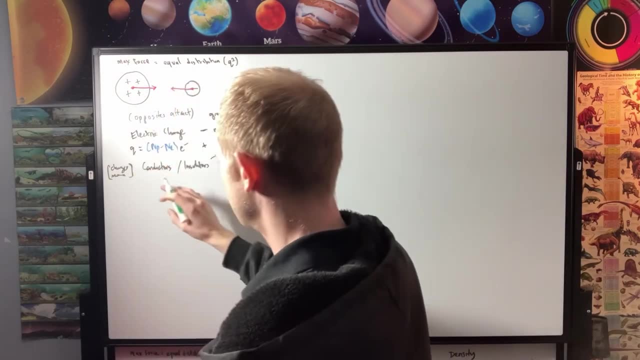 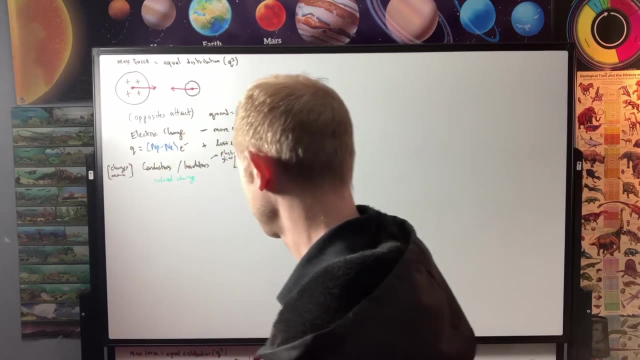 So that means that the charges don't move, They just stay still. That's the main difference. Now there's something that you can do with any kind of material And you can create an induced charge, Induced charge, And so that's basically caused by proximity. 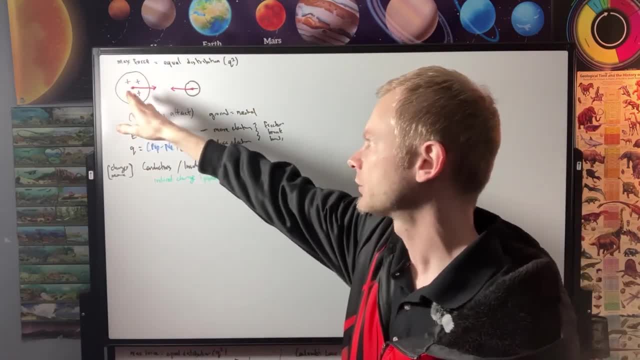 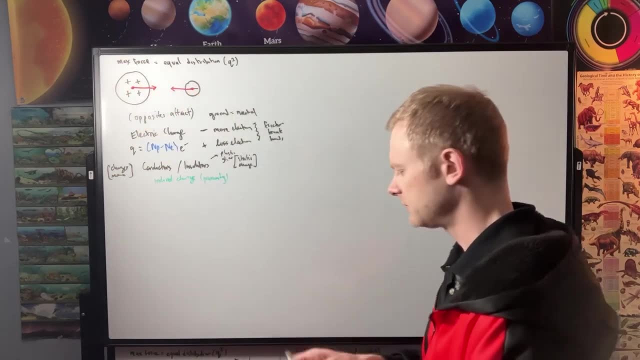 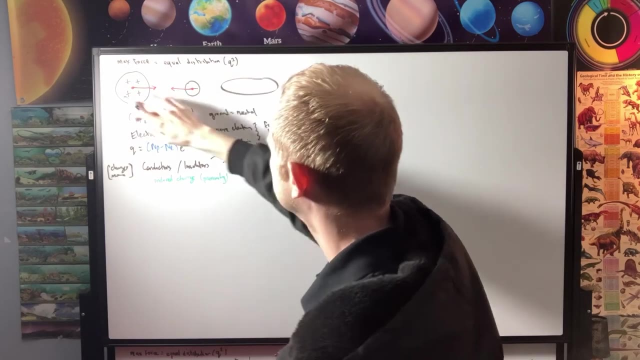 So when you bring like a positively charged object close to- let's say, this was like an insulator and you brought it close to that- it will basically create this thing called a dipole. So here is what a dipole is. You got like say we're bringing this negative thing. 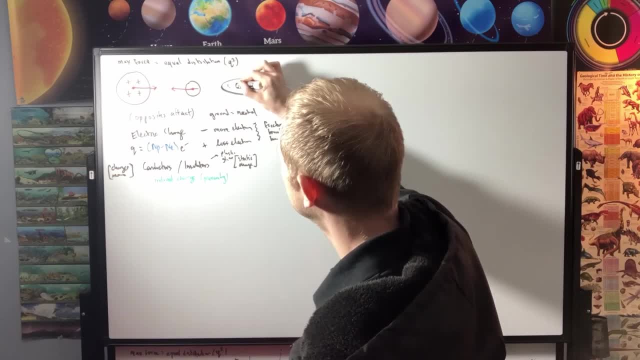 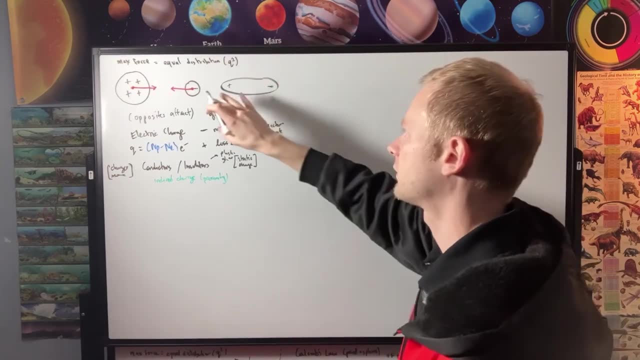 Because the negative is close. you're going to get the positive like charges to like shift over here and sort of move the positive charges over here And the negative charges are going to kind of be repelled and shift over here. This is what a dipole is, because the charges are going to be sort of shifted apart. 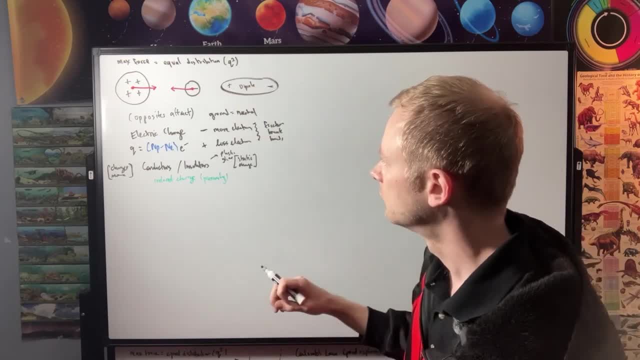 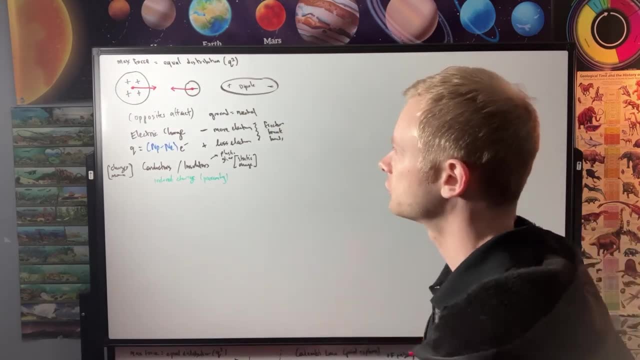 But it's still within that same particle. So you know, you just kind of got like a positive and negative or negative within the same particle, which is kind of strange. It's called an induced charge, usually created by proximity, you know. 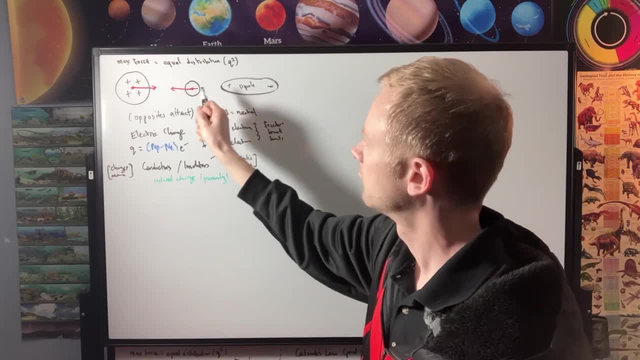 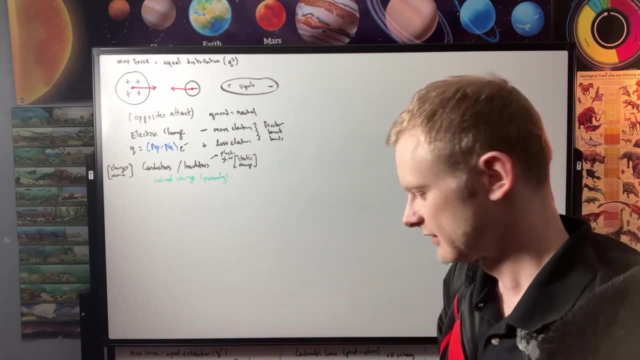 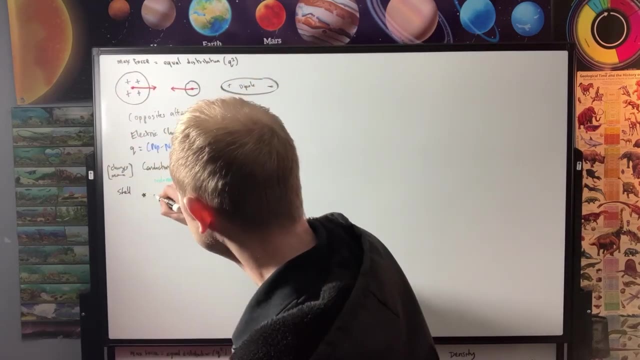 just by having, like, the presence of this negative thing right there is sucking the positives over here and pushing the negatives over there. It's kind of interesting. Now we also have this shell theory idea, The shell. We have to consider this shell. Just realize that anytime you got like charge. 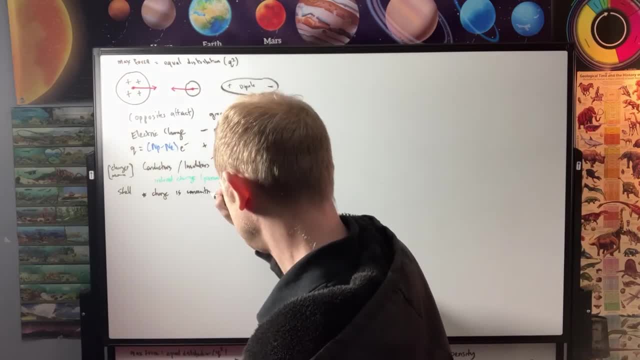 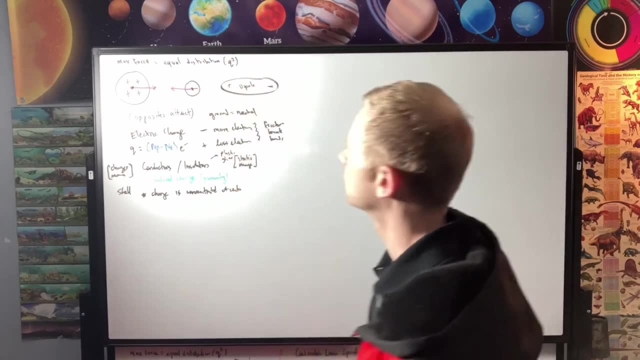 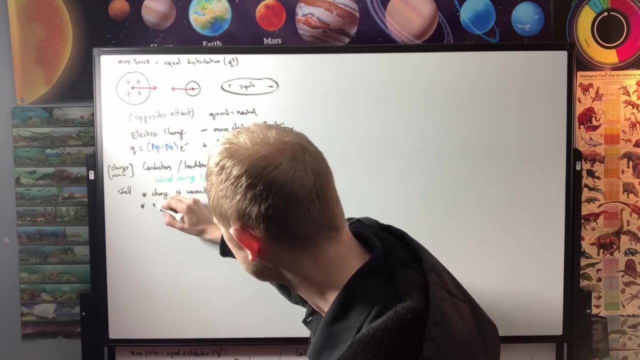 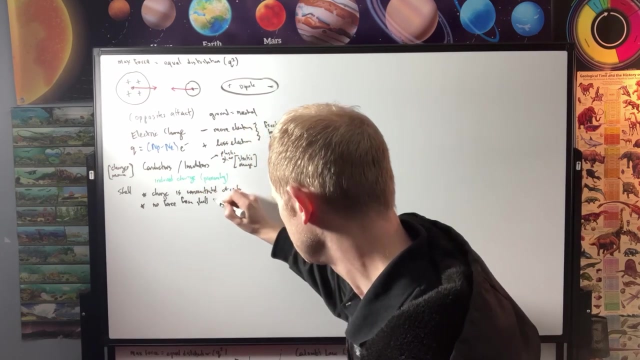 it's concentrated in this center, concentrated at the center, And so that's why they come directly from right here. All right, And another thing is that, no matter where you are, there's never going to be any kind of force from the shell on the inside. 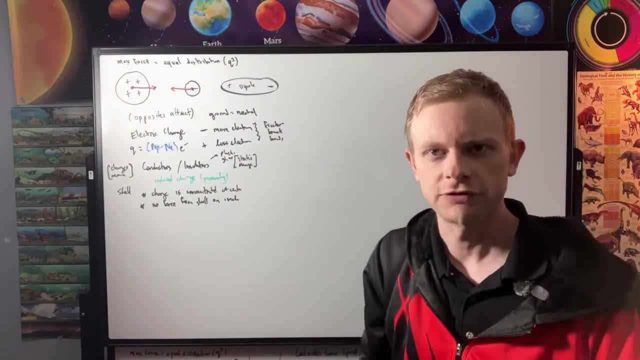 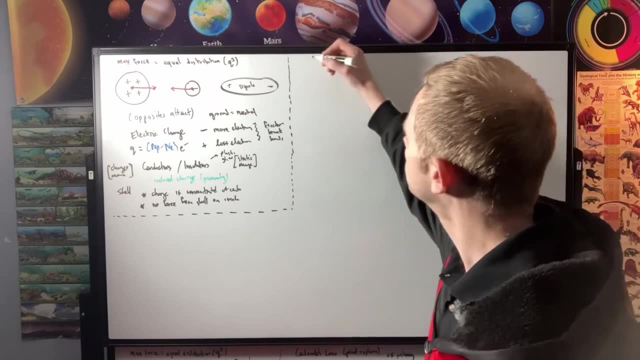 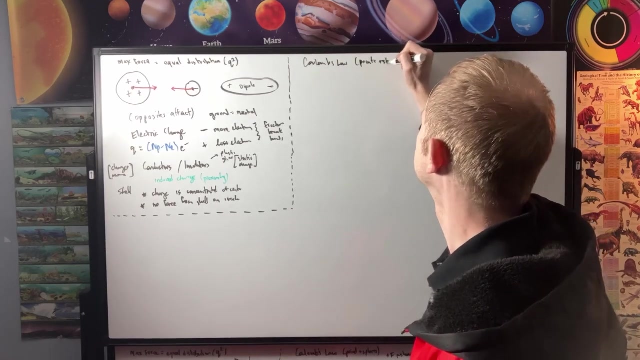 No matter where you are in this particular thing, there's no forces coming, Coming from the shell. So those are the basics of static electricity. Now let's discuss Coulomb's law. Coulomb's law, This is going to work for points and spheres. 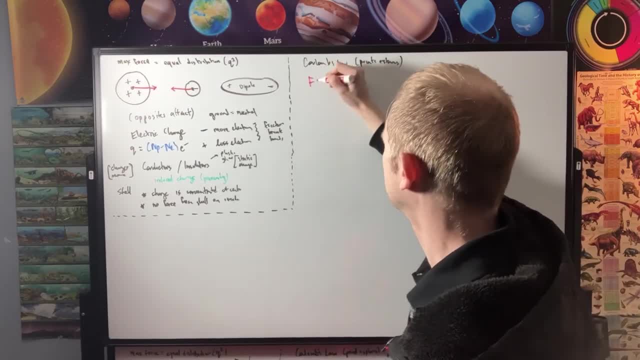 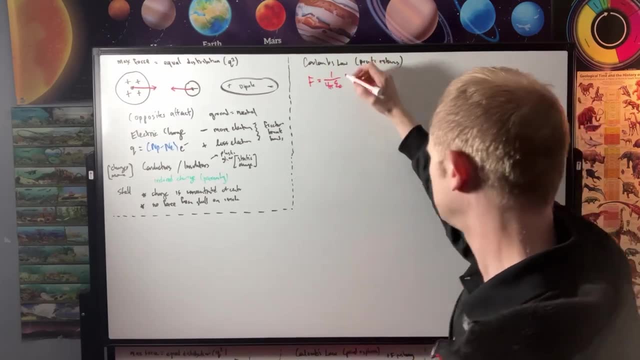 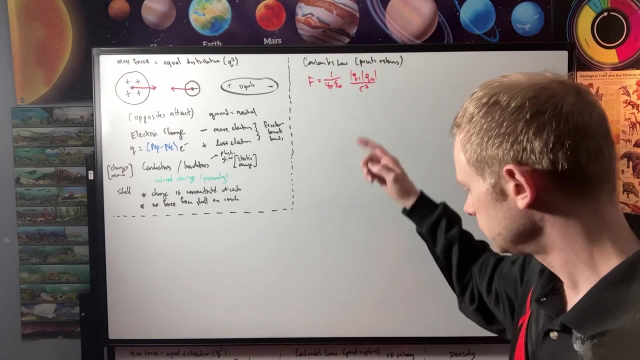 And it's the magnitude of this red arrow over here. So that would be: F equals one over four pi, And then we've got the epsilon knot right there And then we got Q1 times Q2 over R squared. Let's define some of these things here. 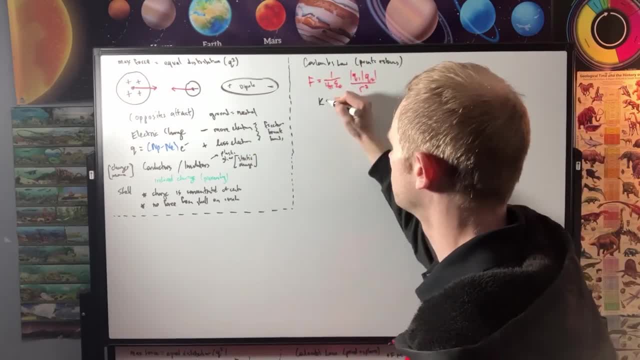 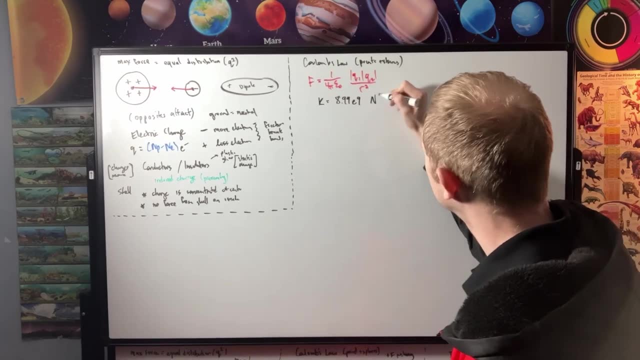 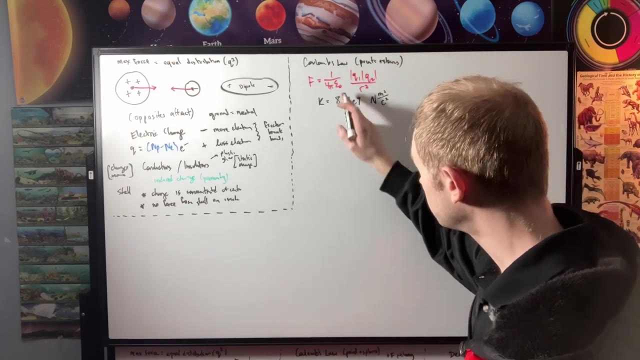 Usually this portion right here is going to be just marked as K. This is 8.99, or just nine times E to the nine And we've got Newton times meters squared over Coulomb squared On this epsilon knot thing right here. this is the permittivity constant. 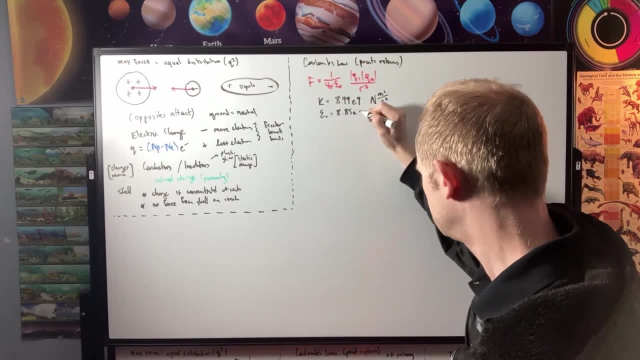 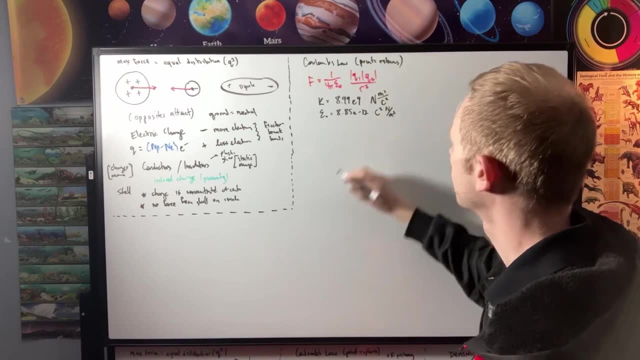 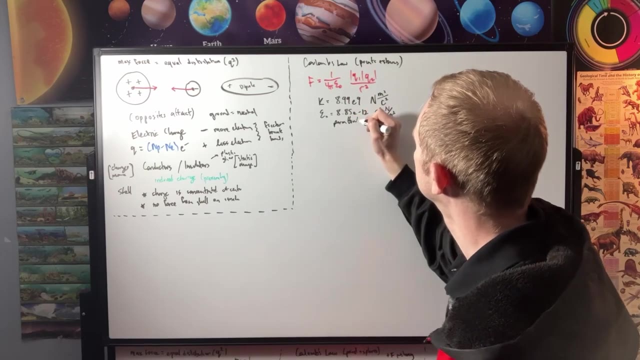 but it's just going to be 8.85 E to the negative 12.. And then Coulomb squared times Newton meters squared, And so yeah, basically, these are just some permittivity, These are just some constants that we have to sort of understand. 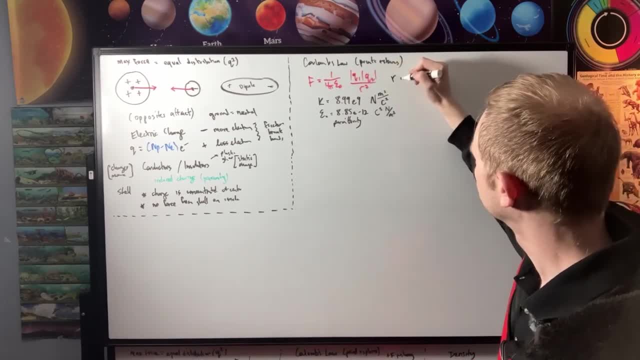 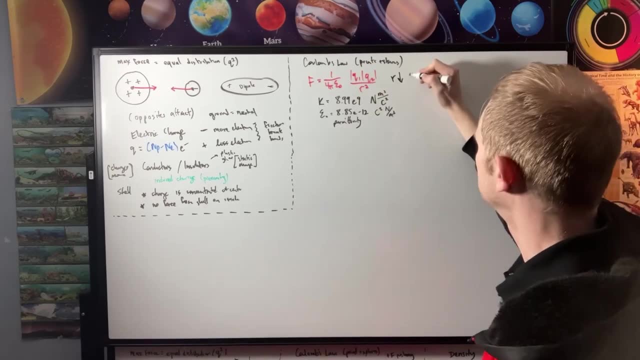 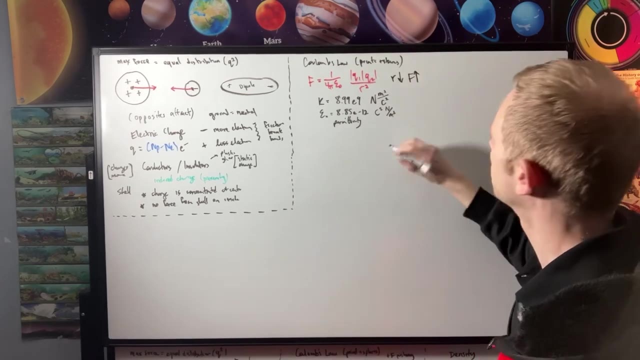 Keeping in mind over here that when we decrease the radius and we pull these two things together, the force is going to increase. So we will mark that right here with this. This will go up as those at this radius decreases, the force increases. 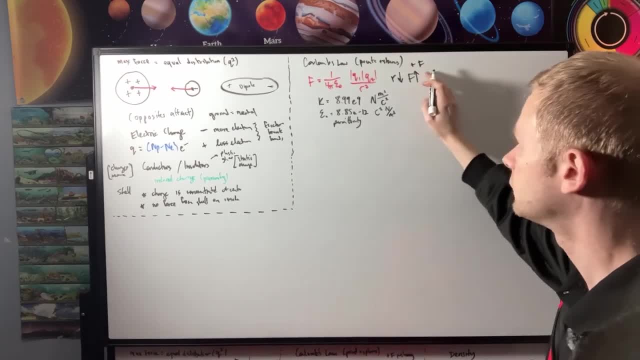 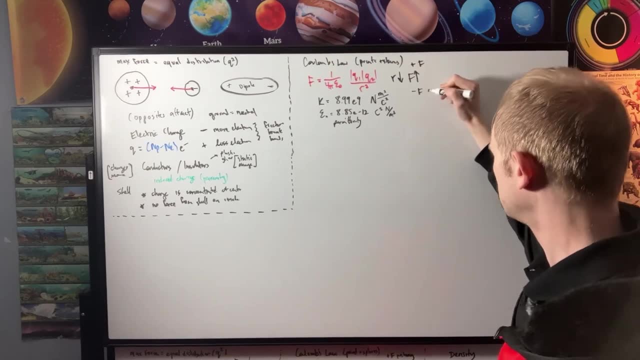 It was marked that over here with, by the way, mentioning that if you have a positive force- remember earlier I mentioned that this is actually a negative force- If you have the negative force, it's going to be pulling, And when you have the positive force, 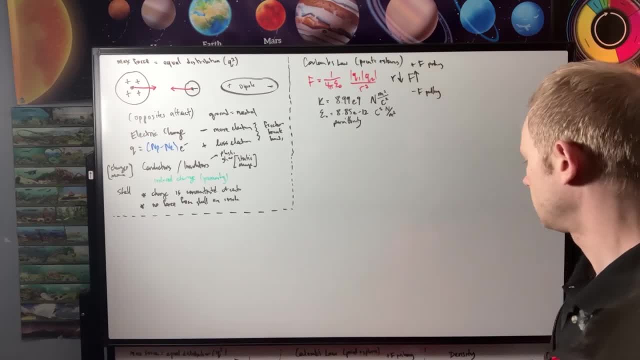 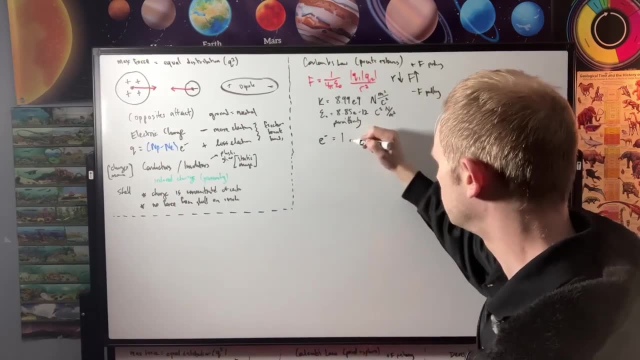 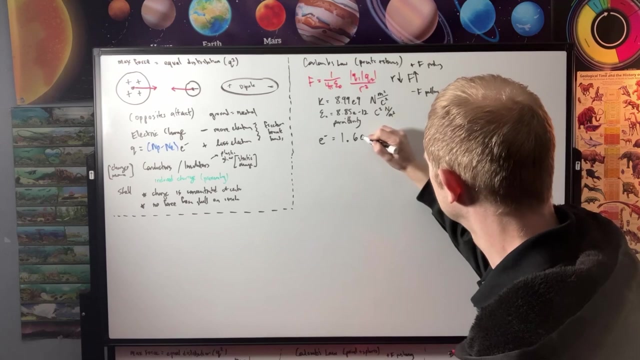 it's going to be pushing. So just keeping those things in mind, And finally, we're also going to define the electrical charge that we said over here. This is the electron charge And we can think of that as the elementary charge. So 1.602 E to the negative 19 Coulombs. 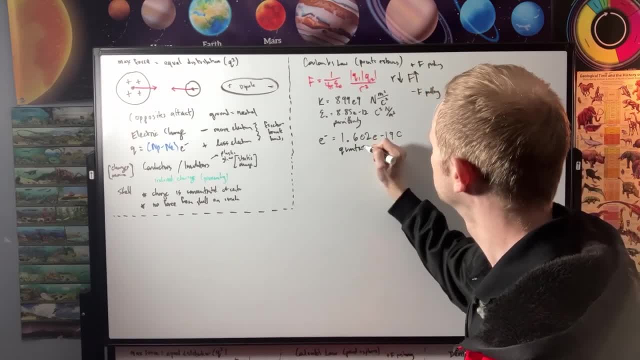 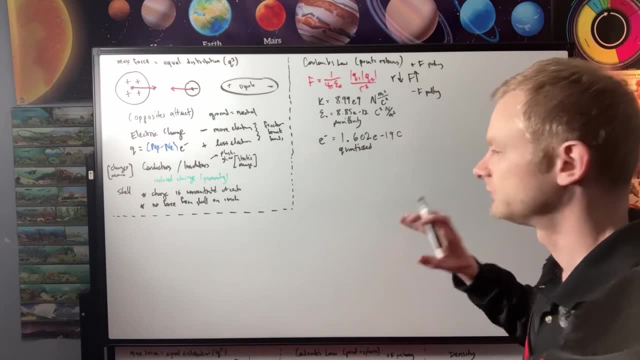 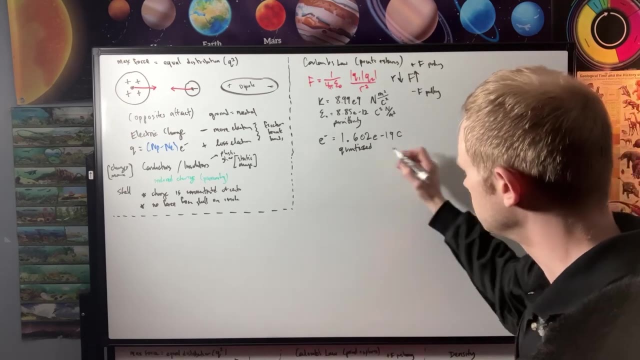 And this is quantized. So the interesting thing about electricity is it's actually quantized, just like light photons and stuff. So it's it's chunks, discrete chunks. There's never going to be half of one of these. This is literally the smallest possible units that you can get. 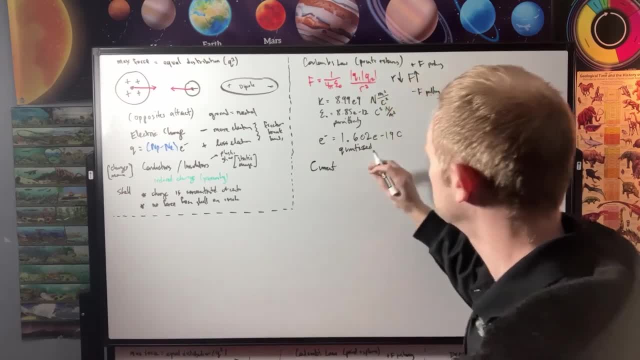 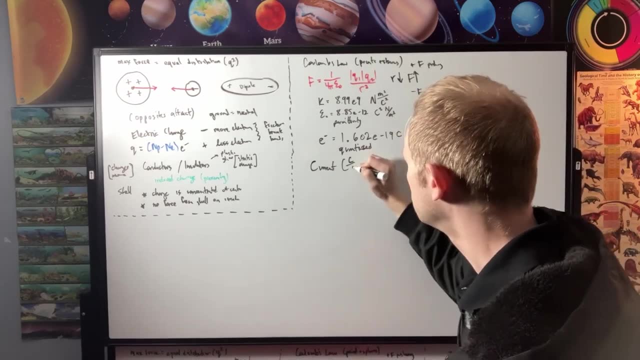 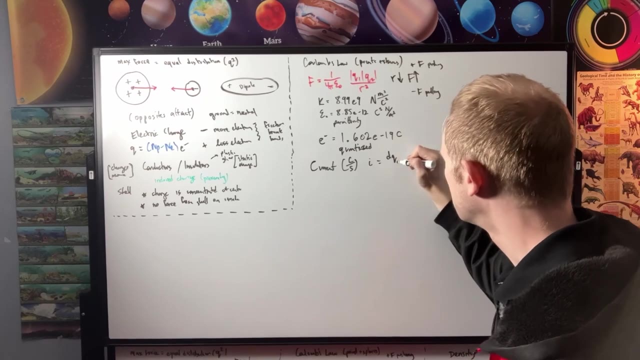 And we also have this thing called current, that you might have to calculate which would be the flow of charge in one particular spot, And let's say that would be Coulombs per second for that one particular point, And so you would have: I equals DQ over DT. 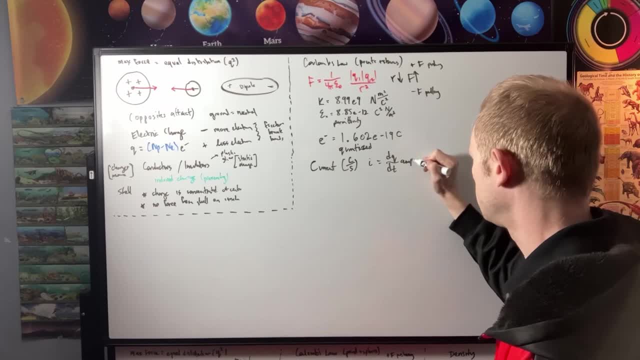 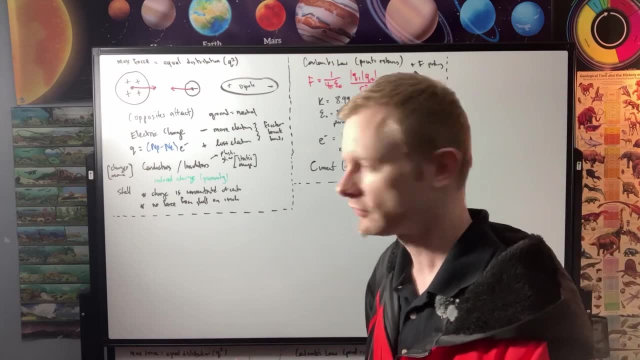 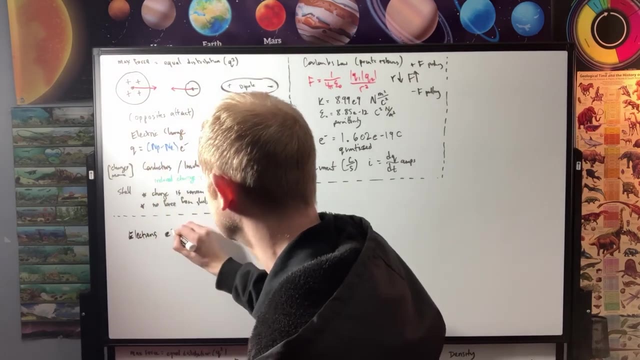 the Coulombs per second, And this is labeled as amps. Interesting. Let's review the basic composition of these particles. Usually there's going to be electrons, And those are marked as E minus. And then we would have protons. Those could be labeled as a P. 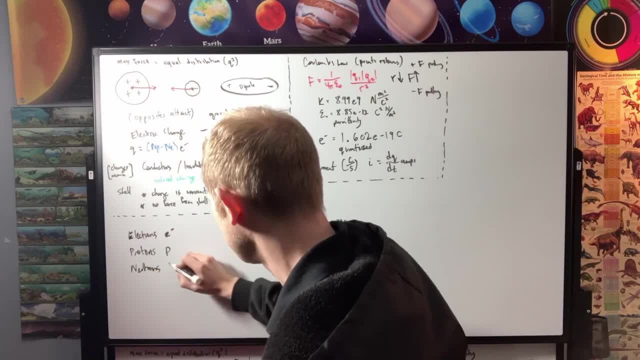 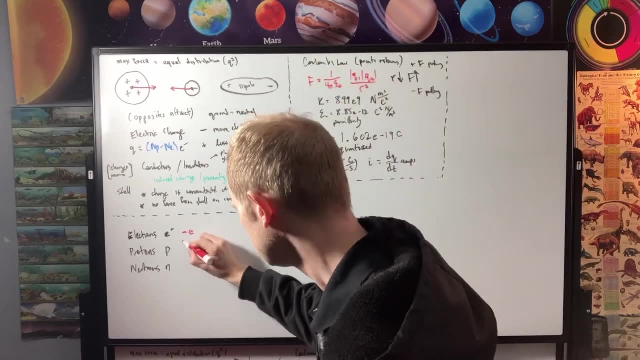 And then we have neutrons, And those are labeled as an N, And then these electrons are going to have a negative. They're going to have a negative elementary charge. The protons are going to have a positive elementary charge And the neutrons have a zero charge. 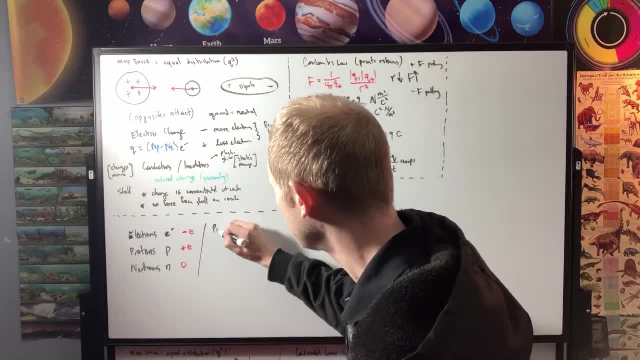 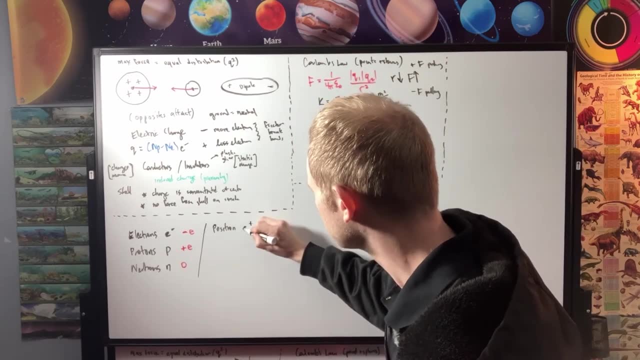 Now let's discuss some antimatter. So let's say we had a positron That's going to be the anti-electron of the century And that is going to be E plus. We'll discuss how we can actually create antimatter a little bit later with radioactive decay. 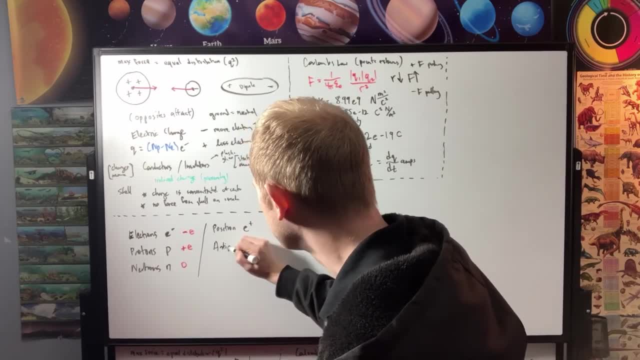 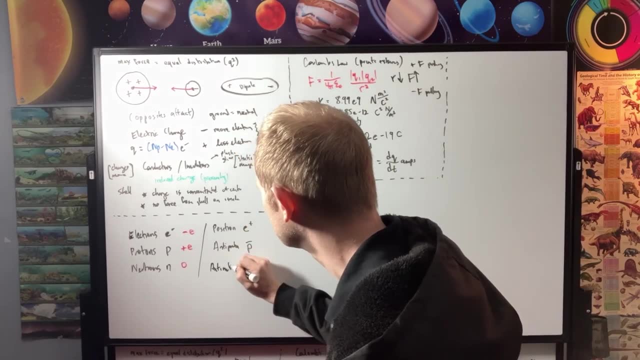 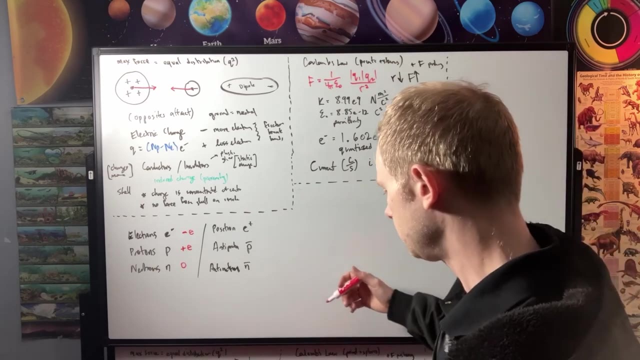 And then we also have the anti-proton, Which would be labeled as P bar, And then we also have the anti-neutron: Anti-neutron, Which is going to be little, with N bar, And well, these are going to have just the opposite charges. 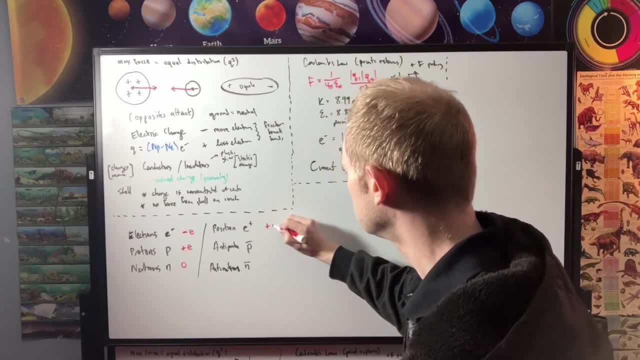 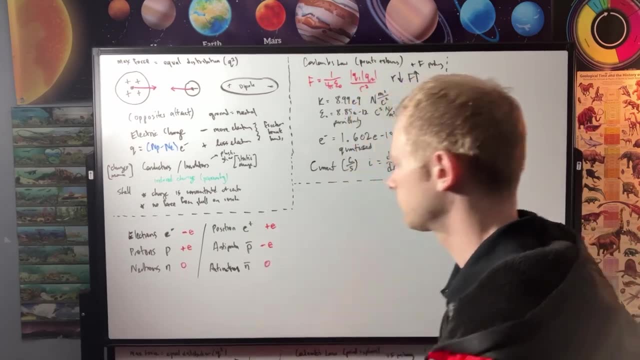 So I mean, that kind of makes sense. It's the anti-particle is going to have the opposite charge, So this would be the proton with a negative charge. And then here we have the neutron, Anti-neutron being zero as well. Antimatter. 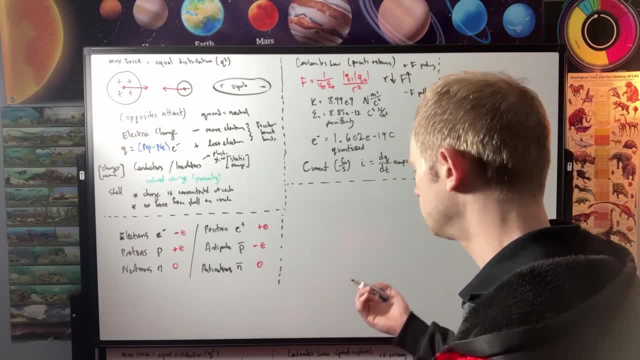 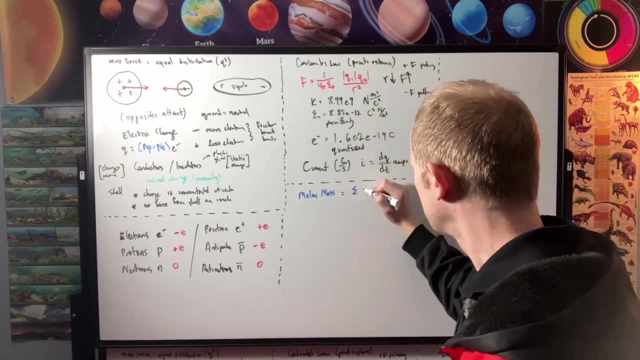 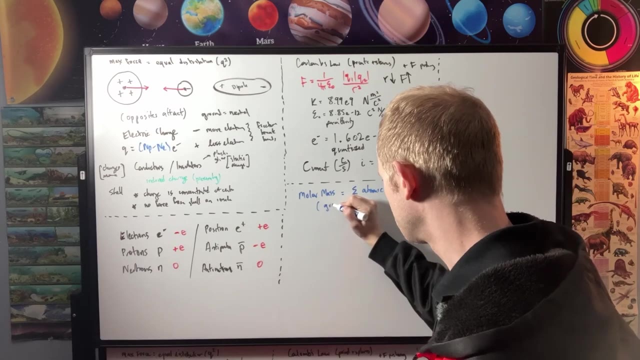 We're going to have to get a little further into chemistry Because some of these problems we're going to have to deal with molar mass. So molar mass is basically the sum of the atomic masses in an element, And so this would be the number of grams in one mole. 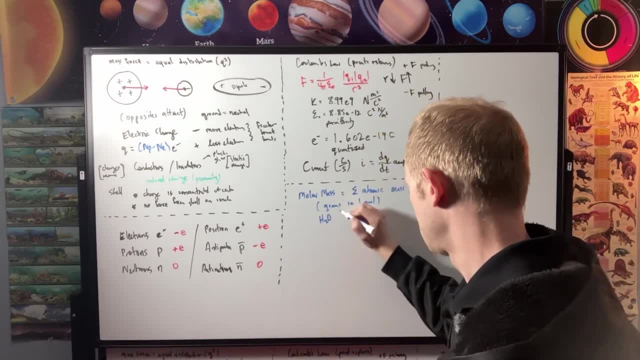 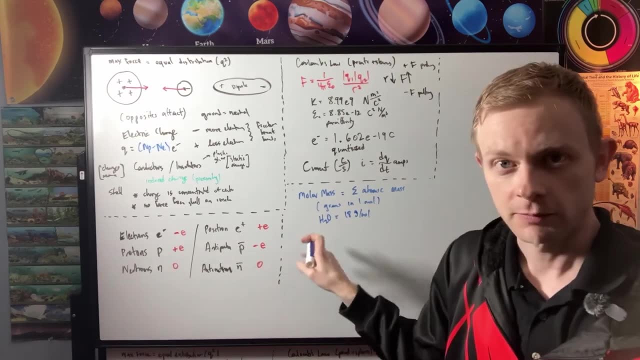 Okay, Let's say we had H2O. We know that that's 18 grams per mole Because the H's on the periodic table are one atomic mass And the O is 16 atomic mass. You can see that on the periodic table. 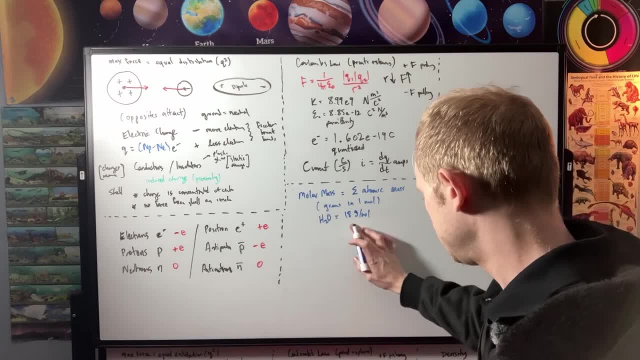 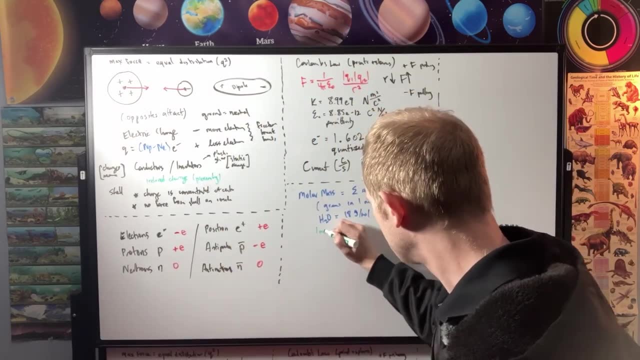 It's not the atomic number, It's the atomic mass. Alright, And one very important thing: Once we've figured out how many moles we have, When we figure out the moles, We've got to figure out how many atoms we have with Avogadro's number. 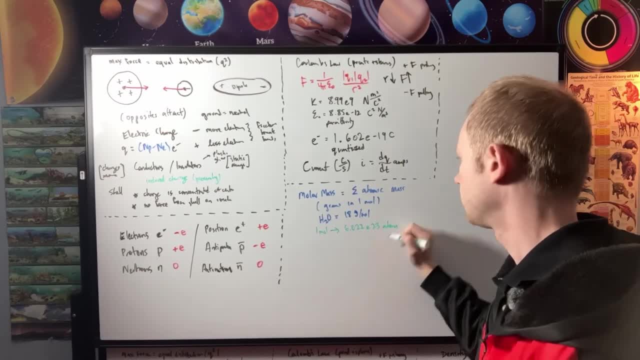 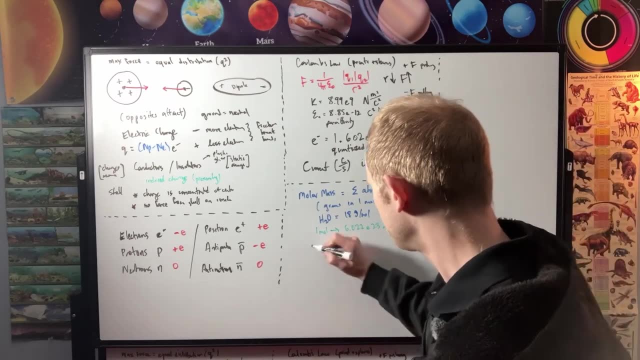 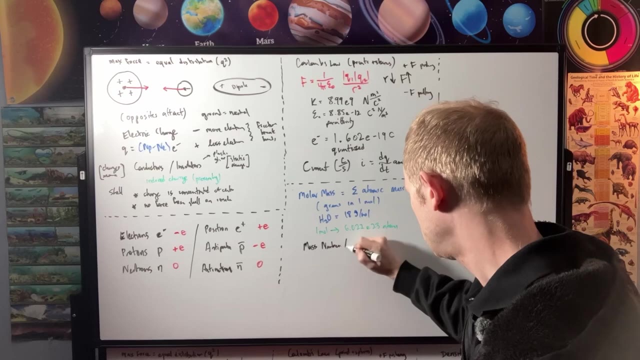 Sometimes we need to do something like this. So when you figure out the moles, Multiply that by the Avogadro's numbers. It will get you how many atoms you have. Some other things: Mass number- That's going to usually be represented as A. 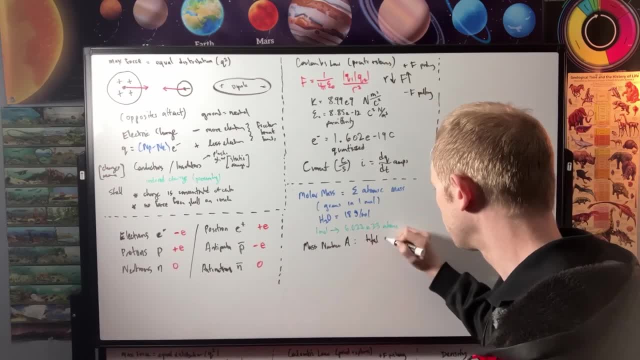 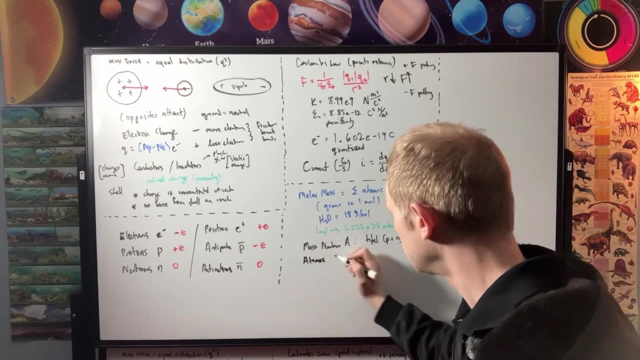 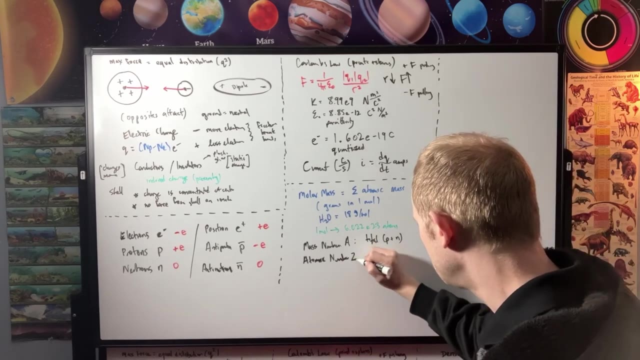 And that's going to be the total number of protons and neutrons. Mass number And then atomic number. This is probably the most important number. Besides, more mass Or atomic mass Is Z. This is the number of protons. 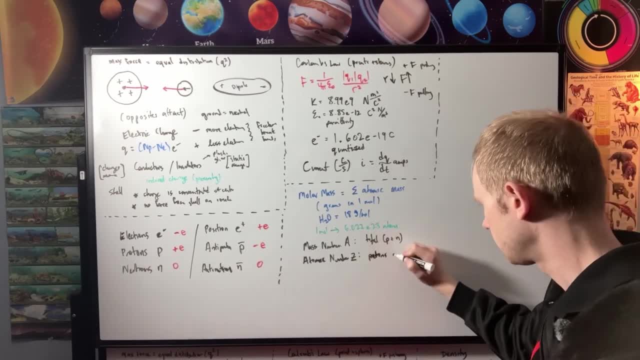 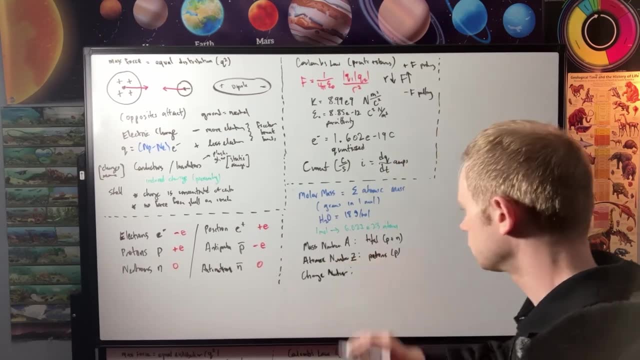 So this is usually how you would find items on the periodic table: By the number of protons P, And let's see Charge number. Okay, Charge number would be like protons minus electrons. Remember the one that we had over here? 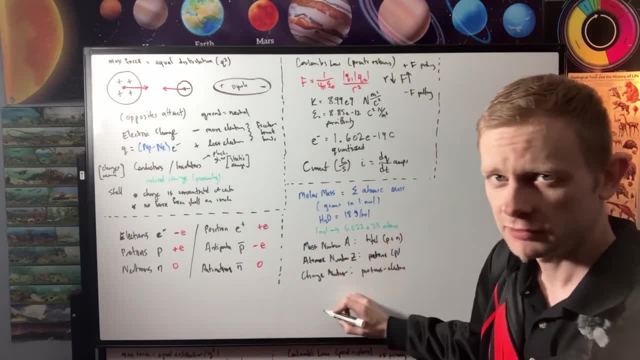 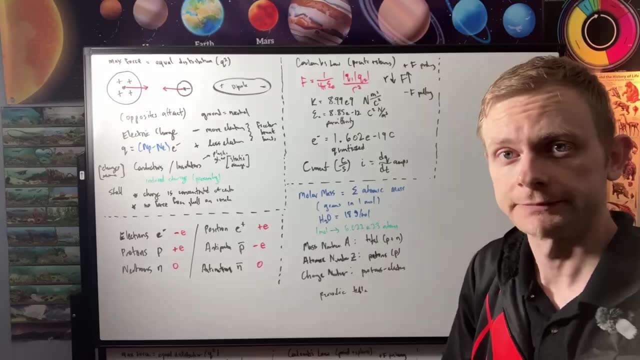 That would be your charge number And I do recommend having a periodic table Just to Just so that you have the periodic table with you. It's pretty important. Density can be a little bit confusing Because there's three kinds of density. 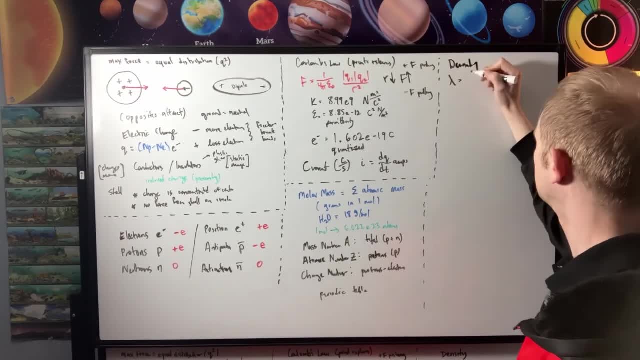 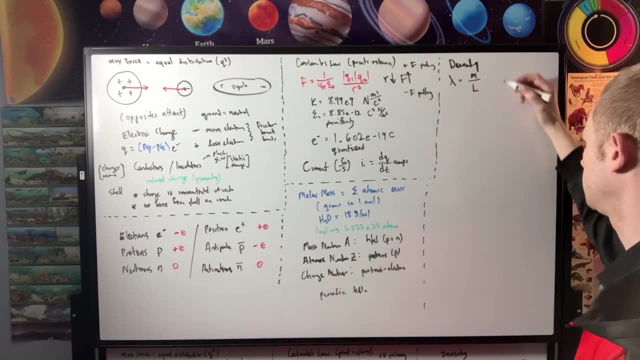 But let's review this. We have the lambda being equal to M over length. So if this was just one dimension, You could figure out what the density is. But if you have two dimensions, That would be M over A, Which is the area. 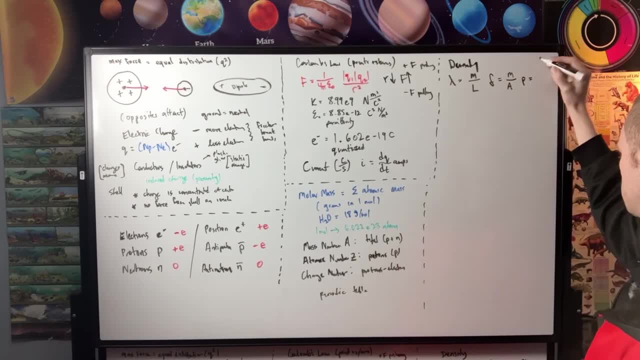 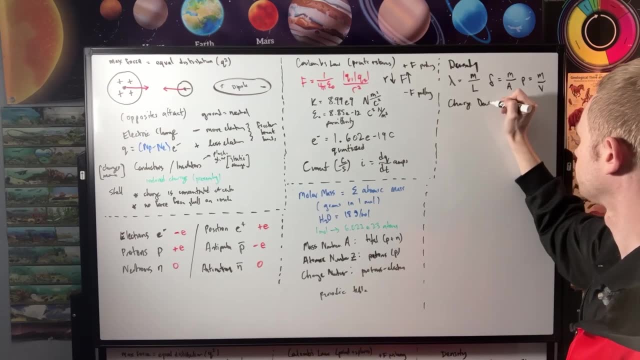 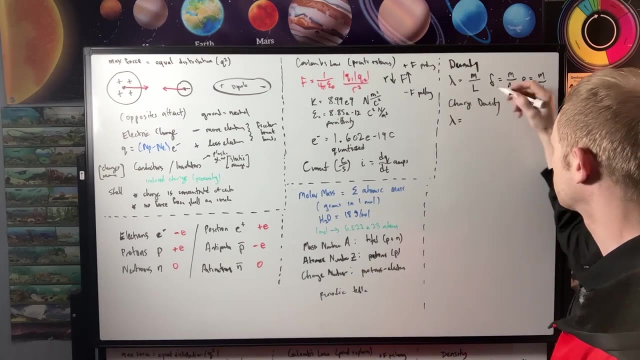 And then If you have three dimensions, That would be P, So M over the volume, Alright, But let's say we wanted to figure out what charge density was. If this is in terms of static electricity and stuff, Well, That would be the same letters here. 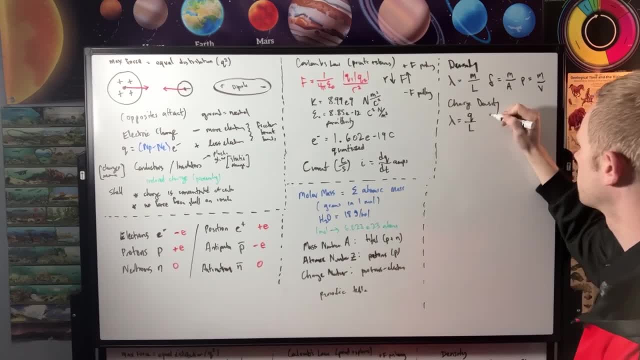 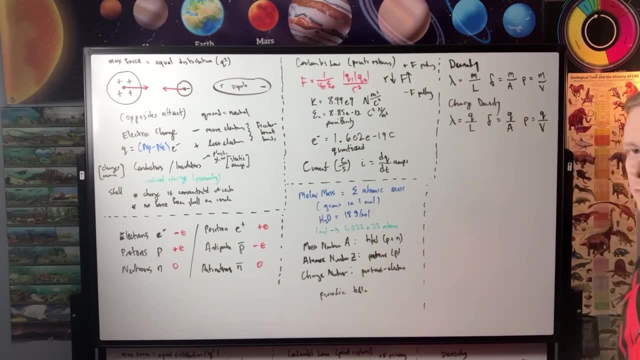 But instead of using mass, We're going to use charge over length, And we're going to use charge over area, And then we're going to use charge over volume In 3D cases. Now, radioactive decay has always been pretty fascinating for me. 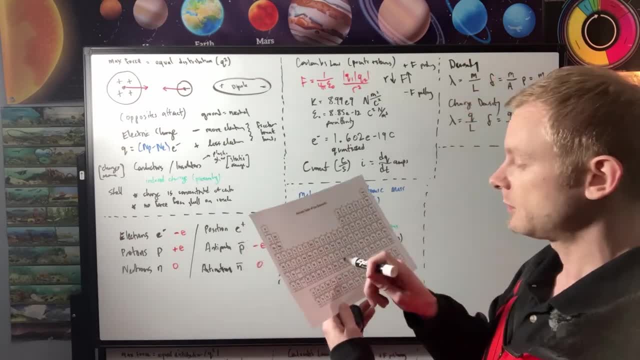 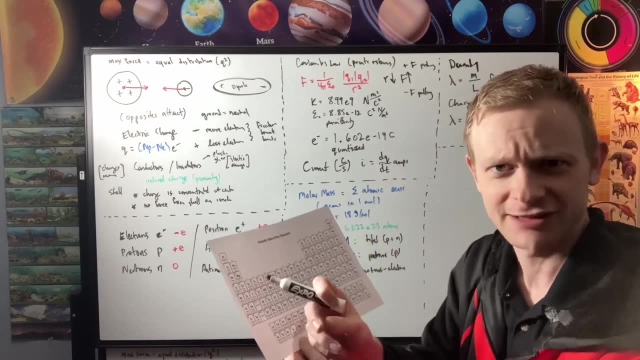 Because basically what it means is You got, like an element on the periodic table And then all of a sudden it just Poof, Turns into the next element. Poof, It just turns into the next element. Poof, Just like that. 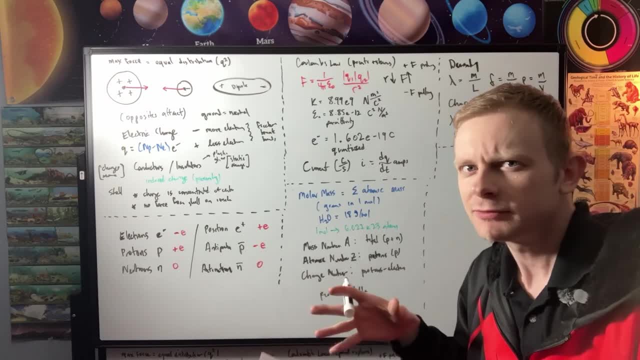 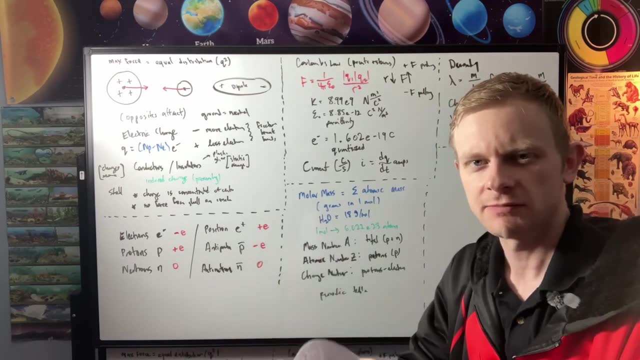 Just like magic. There's like a few ways you can kind of do that In the world, Like you can use gravity Or some mad force amounts And smash things down And basically turn them into the next element That happens in nuclear fusion. 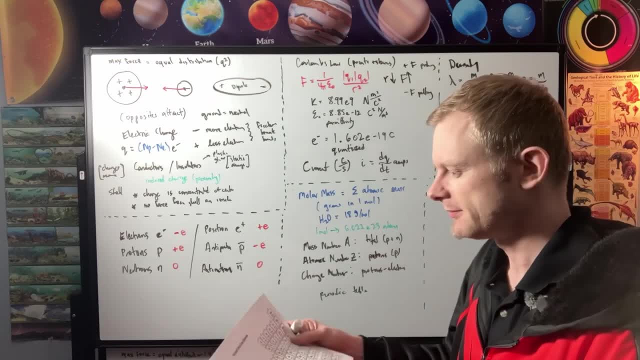 And stars And stuff like that. You might be able to do this with, like Those particle accelerators, Be able to stick some stuff together And create new elements, And the other way is through radioactive decay. So let's define, Let's figure out what that is. 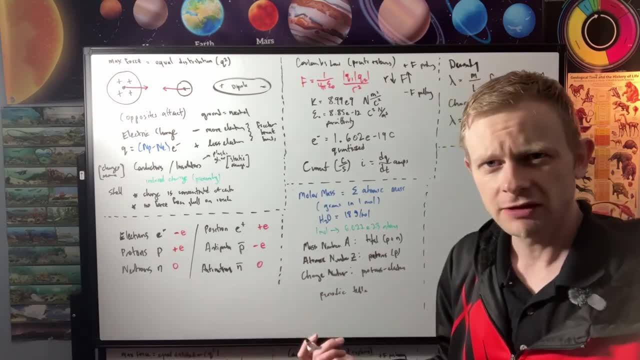 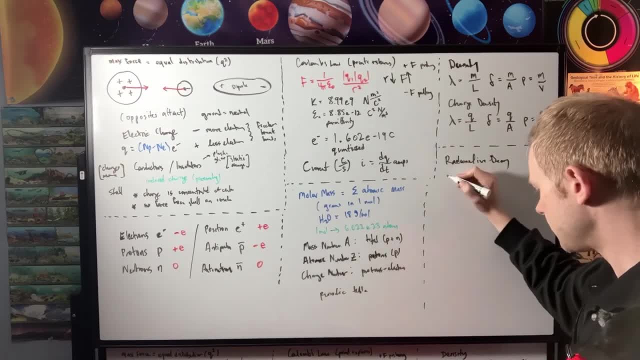 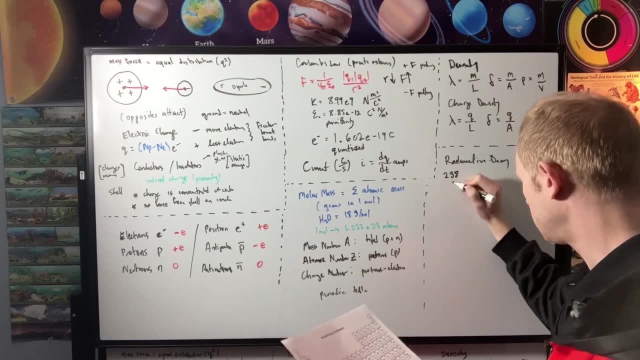 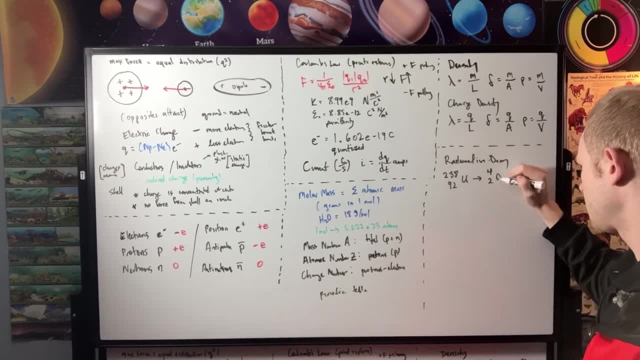 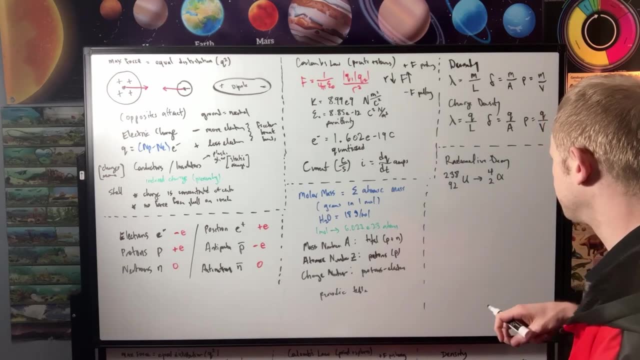 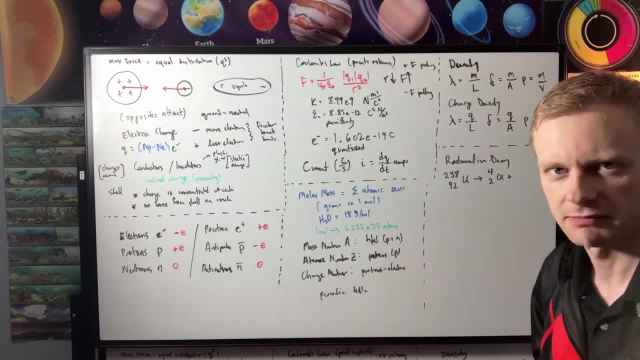 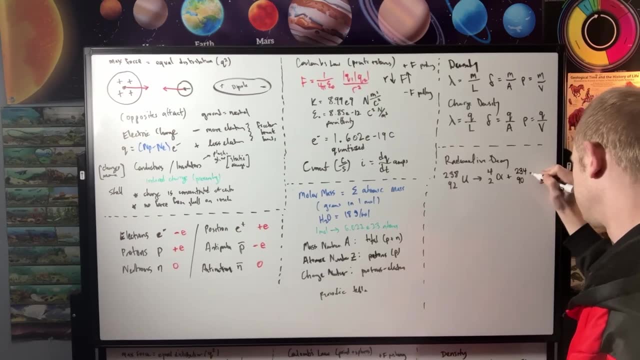 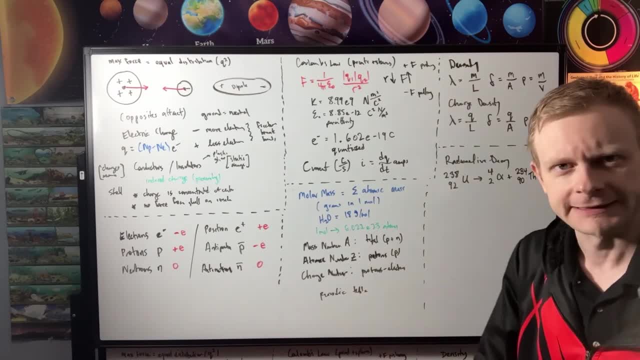 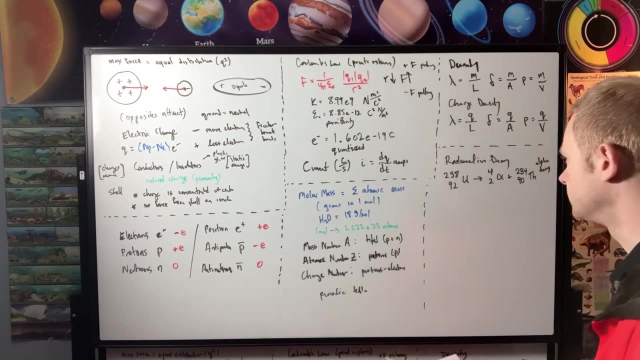 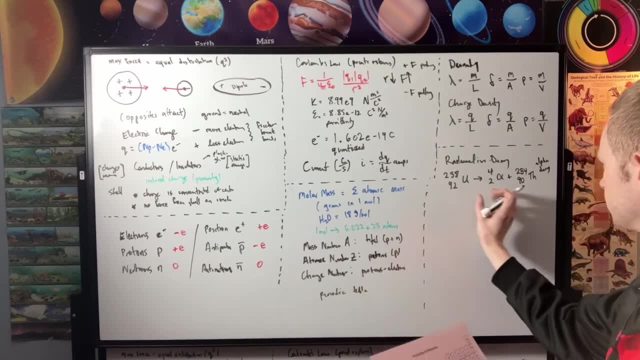 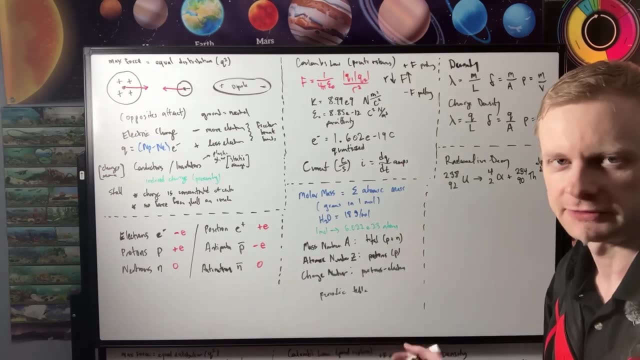 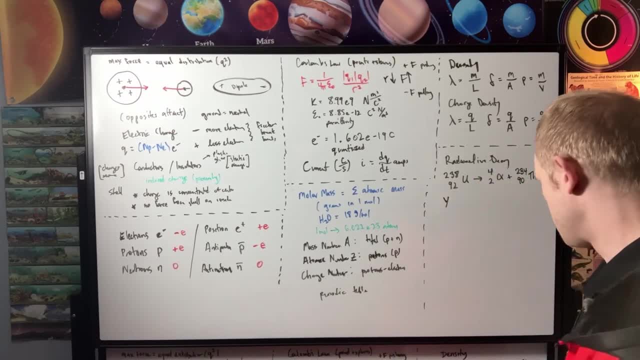 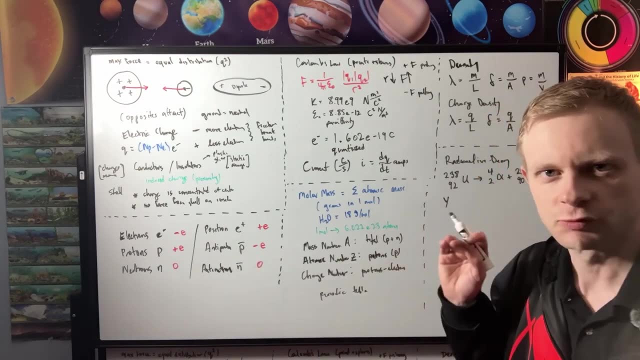 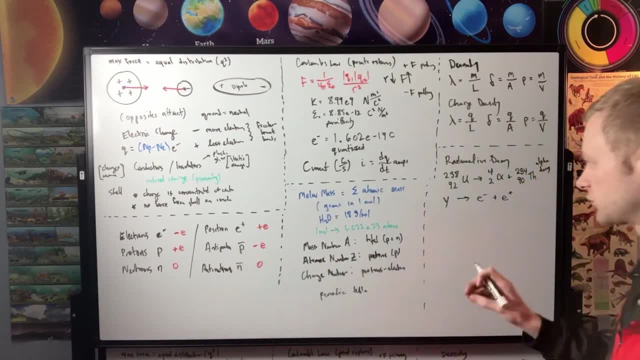 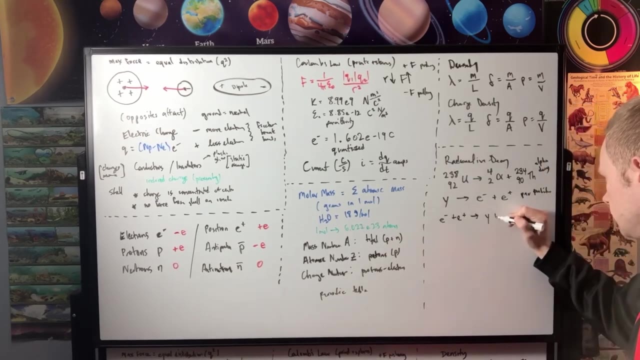 You know, it can become an, an electron and a positron. It can split apart. This is called pair production. pair production. You know this is some crazy stuff as well. You can also have the vice versa happening, but will happen. you'll get two. 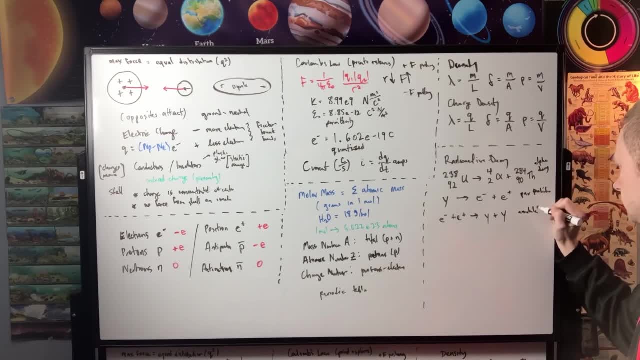 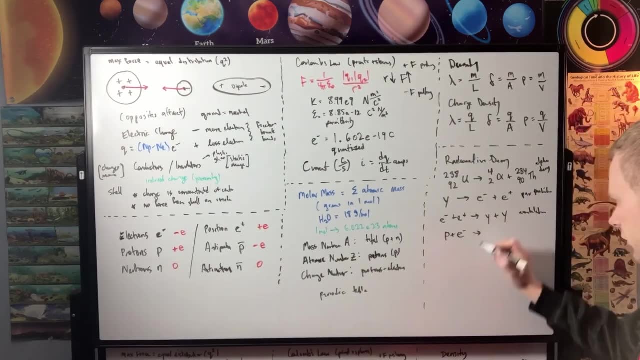 gamma on the other side, and this is annihilation. and And there's also one more that we can kind of take a peek at- it's called electron capture. a proton can eat an electron and Become a neutron and emit a neutrino, and that's called electron capture.